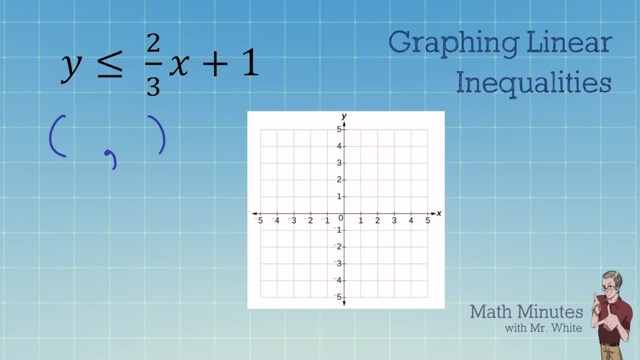 So we're going to try to draw a graph. We're going to draw a graph that shows where all these solutions lie. First order of business is to graph what's called the boundary line, and that's where you replace the inequality with an equal sign and you graph the linear function. y equals 2 thirds x plus 1.. 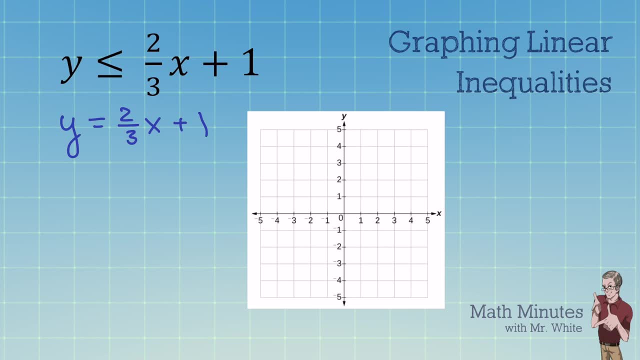 Now you've gotten really good at y equals mx plus b graphing, I imagine. so this should be pretty easy. You go up 1 and put a dot and then the slope is 2 thirds. So from that dot we go up 2 over 3 and put a second dot. 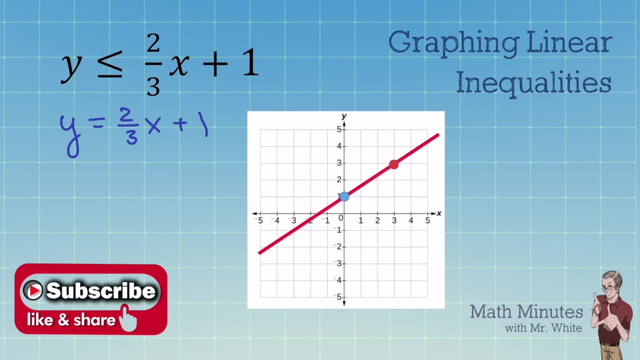 Now We're going to draw a solid line, and I'll get to that in a second why we're drawing a solid line here. Now we have to decide whether to shade above this boundary line or below. So let me explain a couple different ways to approach this. 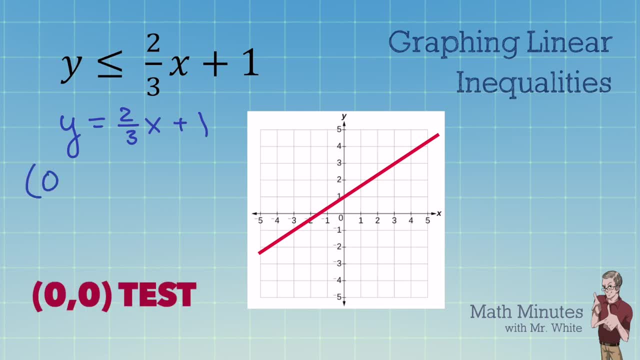 First thing you can do is a thing called the 0-0 test. So we're going to take the point 0-0.. So we're going to plug y equals 0 into our original inequality, and also x equals 0 and see: 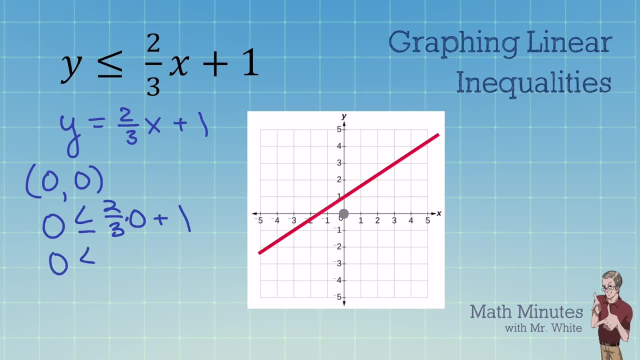 do we have a true statement when we work this out? Is 0 less than or equal to 1?? Well, yes, it is Okay. so the point 0-0 is one of an infinite number of solutions. Now, which side of the line, the boundary line, does that lie? 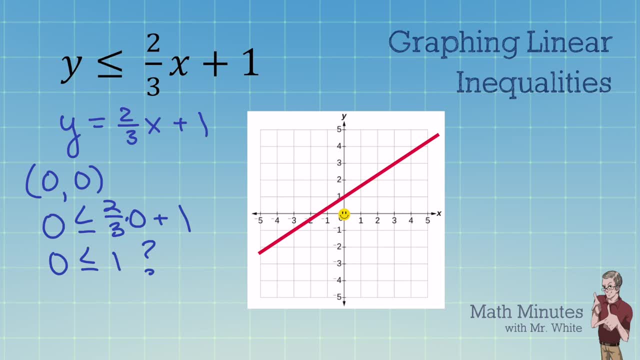 Well, it's underneath the line in this example. right, Sometimes it's over, sometimes it's under, But in this example, that little smiley face I put there because it's a solution is under the line. So where would the rest of the party be going on? 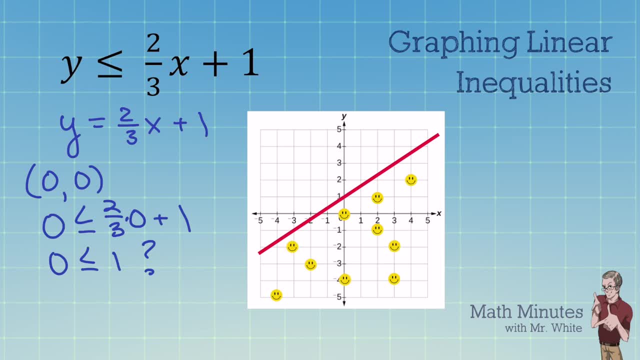 Where are all those smiley faces? They're going to be under the line. So the official graph The official graph is: we draw the line and then we shade below it. So what you see here is the graph of y is less than or equal to 2 thirds x plus 1, and it shows you where all the solutions are. 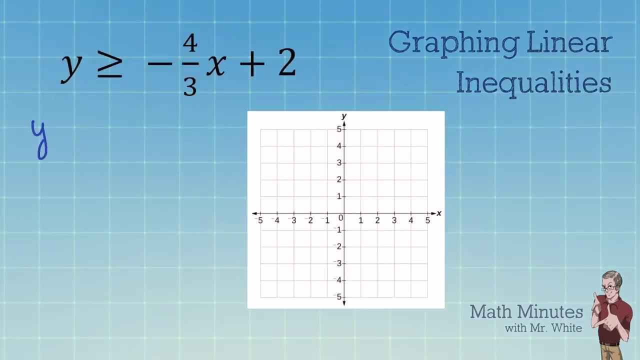 Here in this second example, let's go ahead and graph the boundary line. y equals negative 4 thirds x plus 2, because that's always the first thing you do is graph the boundary line. Now do you see that this is greater than or equal to? 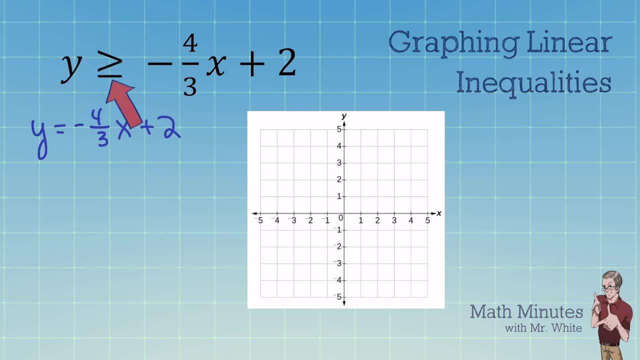 Because it has the equal part to the inequality. that's why we're graphing a solid line, So we're going to do one that doesn't have that equal sign here next. So stick with me and you can learn how to graph those a little bit differently. 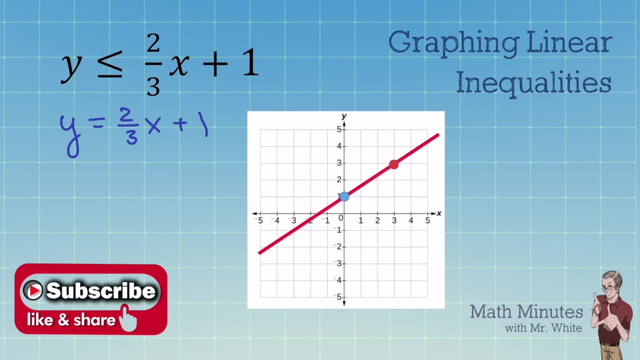 Now We're going to draw a solid line, and I'll get to that in a second why we're drawing a solid line here. Now we have to decide whether to shade above this boundary line or below. So let me explain a couple different ways to approach this. 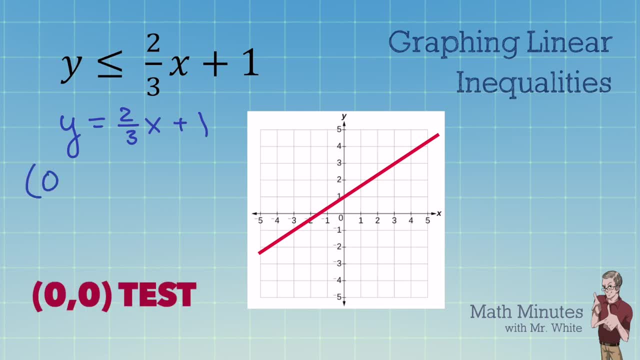 First thing you can do is a thing called the 0-0 test. So we're going to take the point 0-0.. So we're going to plug y equals 0 into our original inequality, and also x equals 0 and see: 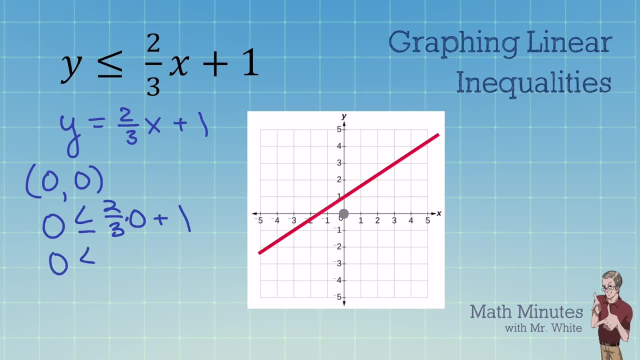 do we have a true statement when we work this out? Is 0 less than or equal to 1?? Well, yes, it is Okay. so the point 0-0 is one of an infinite number of solutions. Now, which side of the line, the boundary line, does that lie? 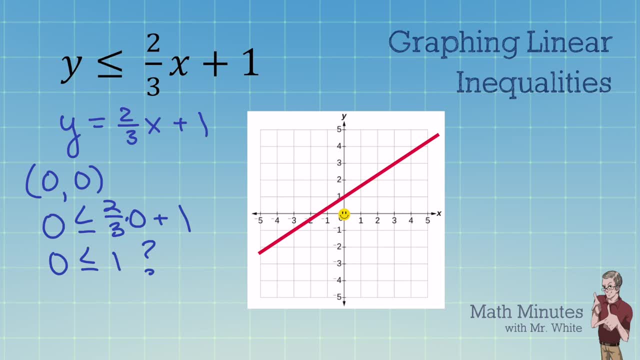 Well, it's underneath the line in this example. right, Sometimes it's over, sometimes it's under, But in this example, that little smiley face I put there because it's a solution is under the line. So where would the rest of the party be going on? 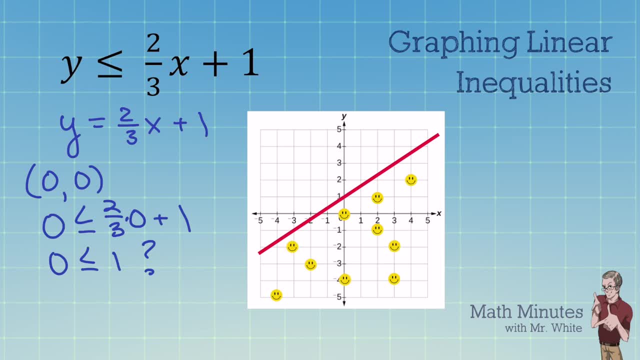 Where are all those smiley faces? They're going to be under the line. So the official graph The official graph is: we draw the line and then we shade below it. So what you see here is the graph of y is less than or equal to 2 thirds x plus 1, and it shows you where all the solutions are. 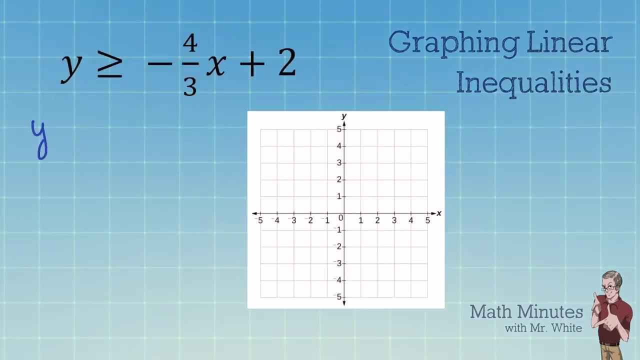 Here in this second example, let's go ahead and graph the boundary line. y equals negative 4 thirds x plus 2, because that's always the first thing you do is graph the boundary line. Now do you see that this is greater than or equal to? 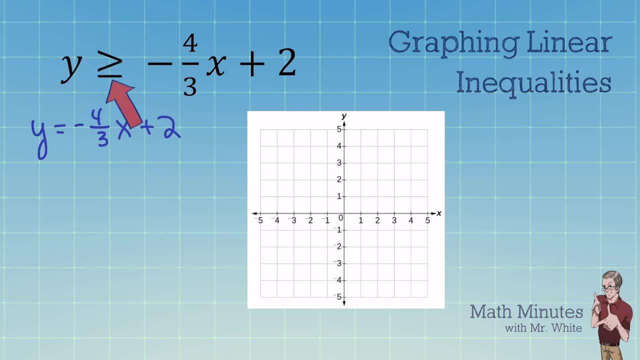 Because it has the equal part to the inequality. that's why we're graphing a solid line, So we're going to do one that doesn't have that equal sign here next. So stick with me and you can learn how to graph those a little bit differently. 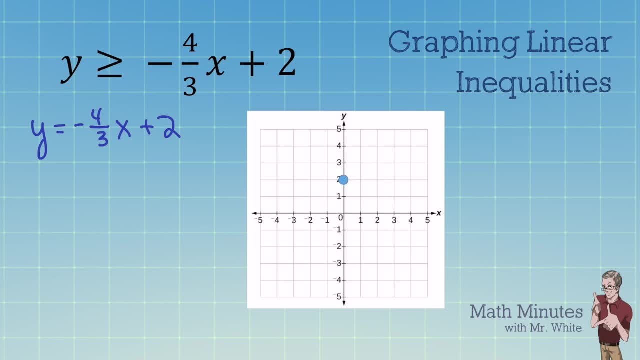 So to graph this boundary line, we go up 2, put a dot and then from there, because the slope is negative, 4 thirds, we're going to go down 4 over 3 to get our second dot. We draw the line. 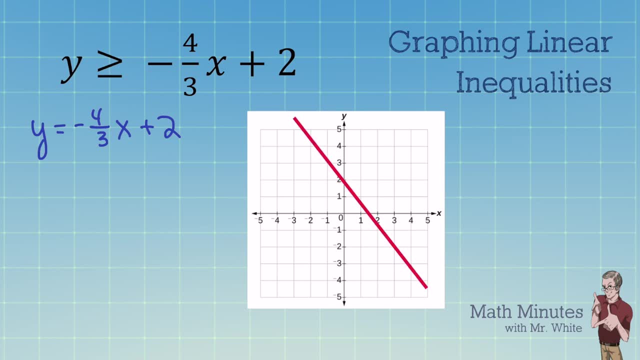 Of course it's going down and to the right because it's a negative slope. So that makes sense. Now we need to figure out which way to shade. So in the last example I showed you the 0, 0 test. 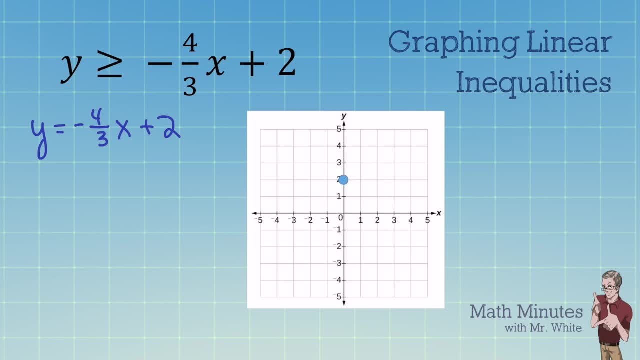 So to graph this boundary line, we go up 2, put a dot and then from there, because the slope is negative, 4 thirds, we're going to go down 4 over 3 to get our second dot. We draw the line. 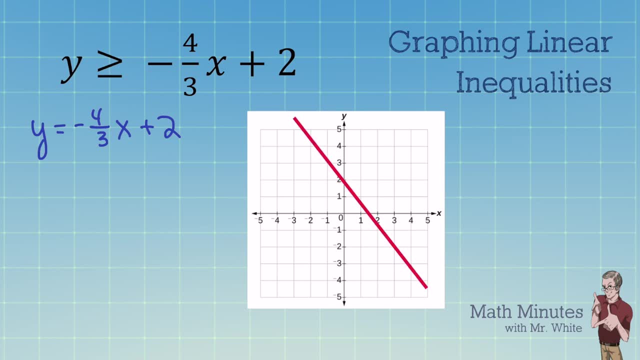 Of course it's going down and to the right because it's a negative slope. So that makes sense. Now we need to figure out which way to shade. So in the last example I showed you the 0, 0 test. 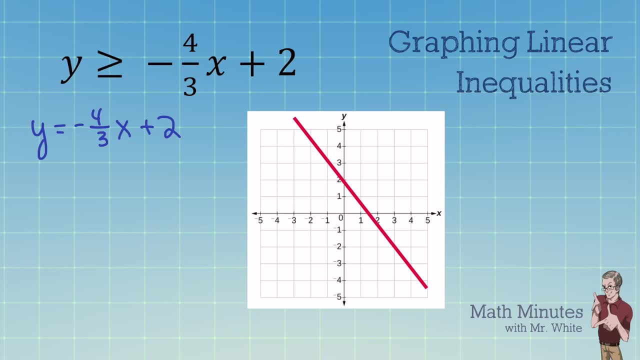 There's another really nice way to graph these And here's how it goes. As long as y is solved all by itself, if you have a greater than, or a greater than or equal to, you're going to shade up. If you have a less than or equal to, 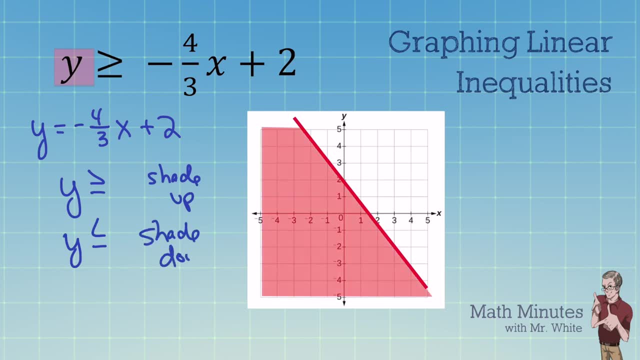 then you're going to shade down under the line. So I don't ever want you to think about left or right, I want you to think about up or down. So anything greater than or equal to, you shade up. Anything less than or equal to. 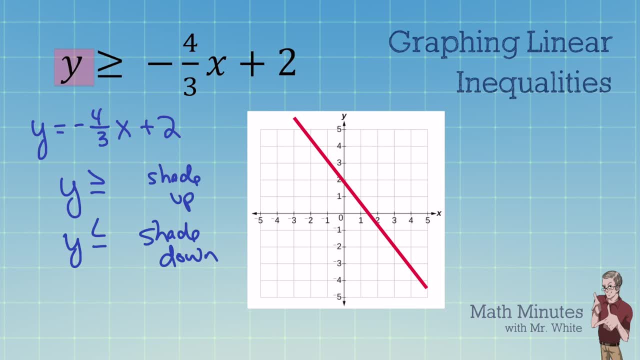 you shade down, And remember, y has to be all by itself in order for that to work. So in our example here, are we going to shade up or down? It looks like y is greater than or equal to. I think we shade up. 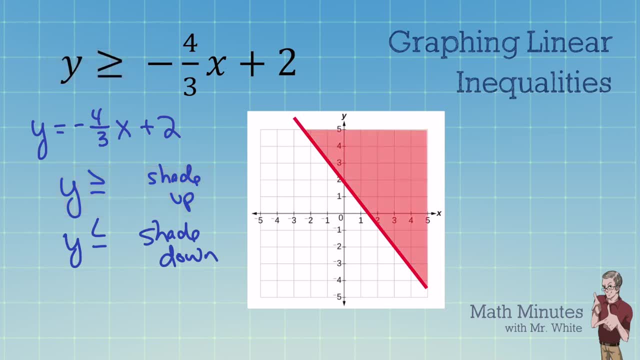 We shade up, We fill it in And there's your graph for the original inequality And it shows you where all the solutions are. So let me ask you this: Is 5, 5 a solution? Well, yes, it is. 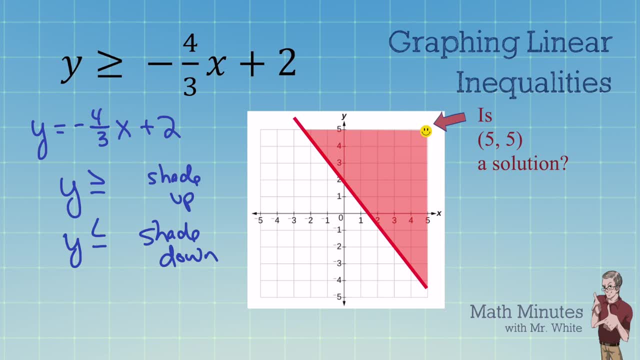 You see how it lies in the shaded region. 5, 5 would be one of an infinite number of solutions. Now, what about negative 5,? negative 5, way down there in the left corner? No, of course not. 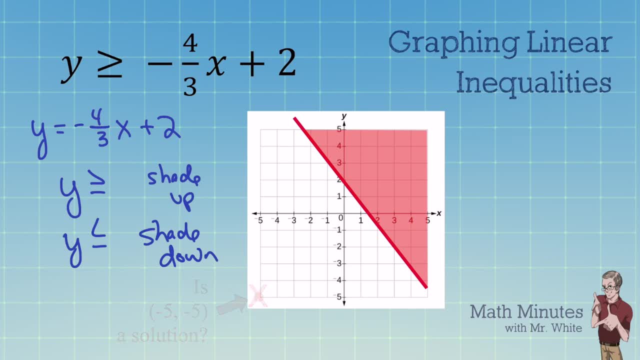 That's not in the shaded region. So you see how this graph shows us where all the solutions are to the inequality. All right, be sure to stick with me, because in this problem we do not have that equal sign right? It's just less than. 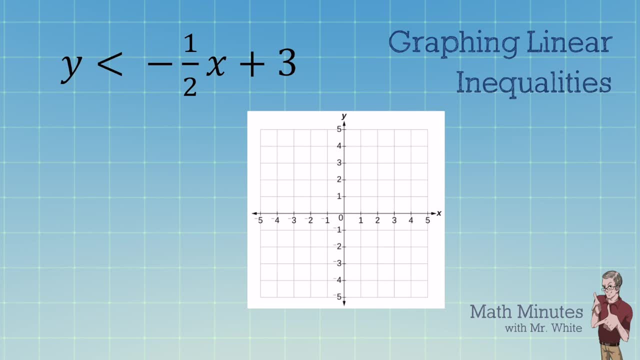 So you're going to see how that graph is different. And then, in the next example, I've got another twist for you that you need to see before you jump into your assignment on this material. All right, so we're going to graph the boundary line. 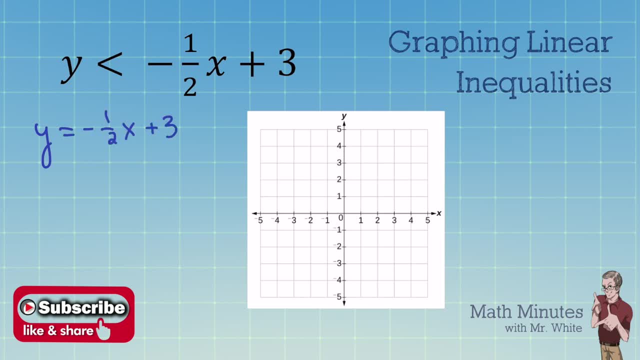 y equals negative 1, half x plus 3.. So we go up 3, put a dot From there, because the slope is negative 1. third, we're going to go down 1 to the right 2 and get our second dot. 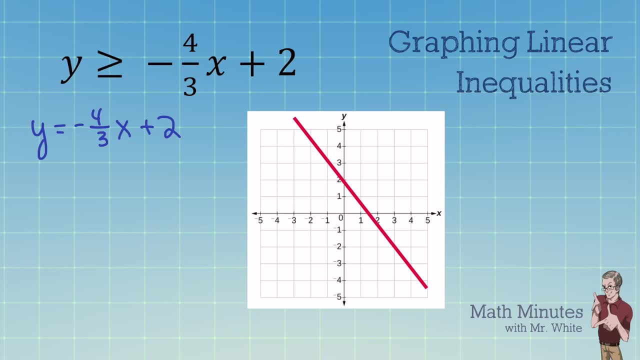 There's another really nice way to graph these And here's how it goes. As long as y is solved all by itself, if you have a greater than, or a greater than or equal to, you're going to shade up. If you have a less than or equal to, 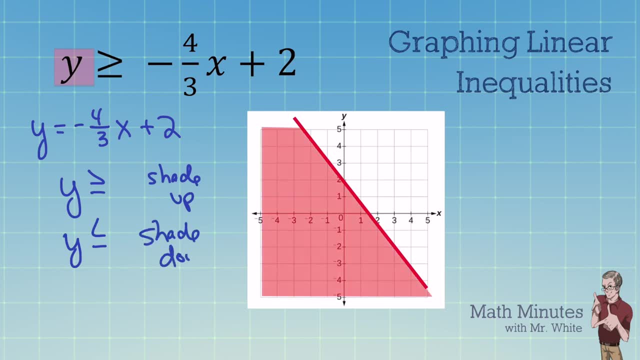 then you're going to shade down under the line. So I don't ever want you to think about left or right, I want you to think about up or down. So anything greater than or equal to, you shade up. Anything less than or equal to. 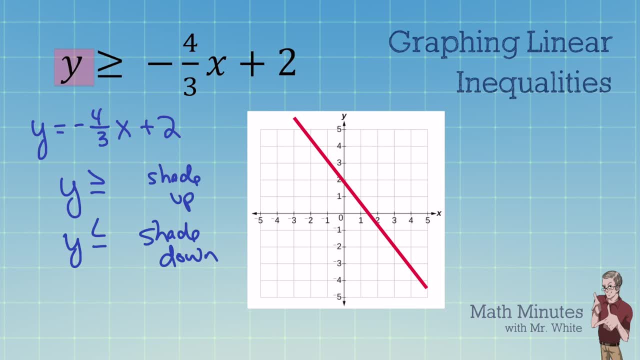 you shade down, And remember, y has to be all by itself in order for that to work. So in our example here, are we going to shade up or down? It looks like y is greater than or equal to. I think we shade up. 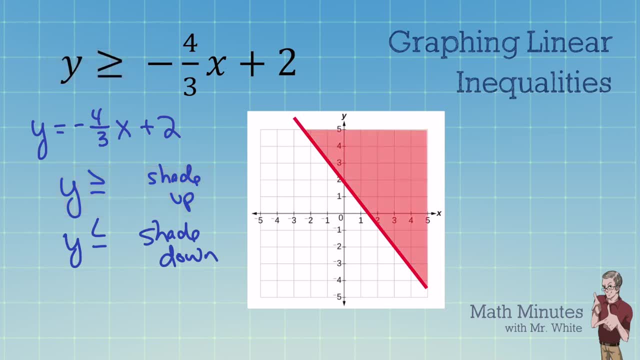 We shade up, We fill it in And there's your graph for the original inequality And it shows you where all the solutions are. So let me ask you this: Is 5, 5 a solution? Well, yes, it is. 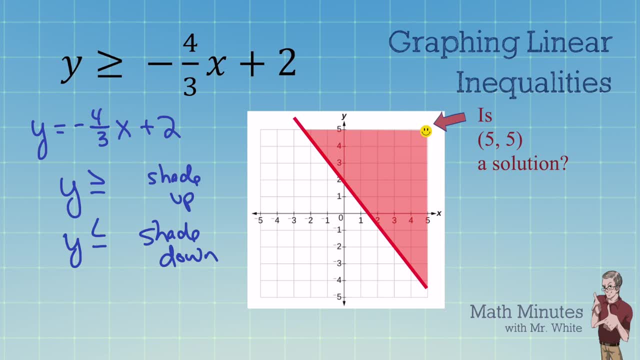 You see how it lies in the shaded region. 5, 5 would be one of an infinite number of solutions. Now, what about negative 5,? negative 5, way down there in the left corner? No, of course not. 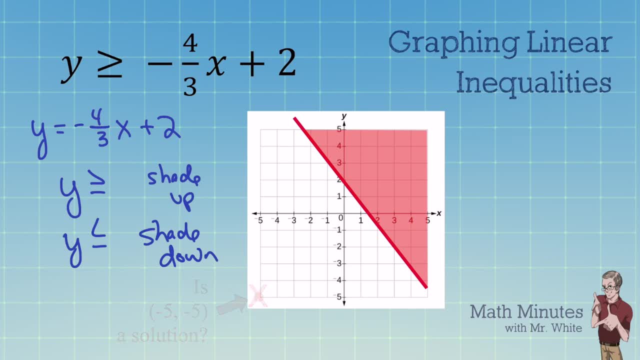 That's not in the shaded region. So you see how this graph shows us where all the solutions are to the inequality. All right, Be sure to stick with me, because in this problem we do not have that equal sign right. It's just less than. 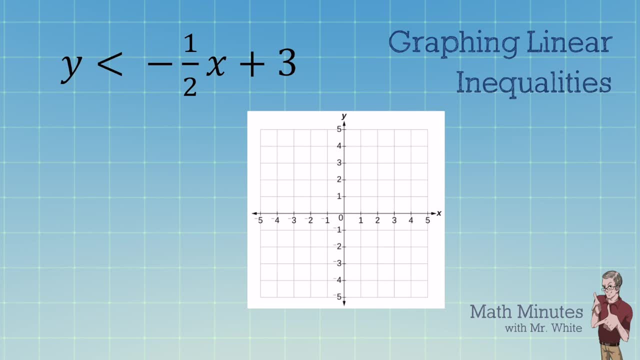 So you're going to see how that graph is different. And then, in the next example, I've got another twist for you that you need to see before you jump into your assignment on this material. All right, so we're going to graph the boundary line. 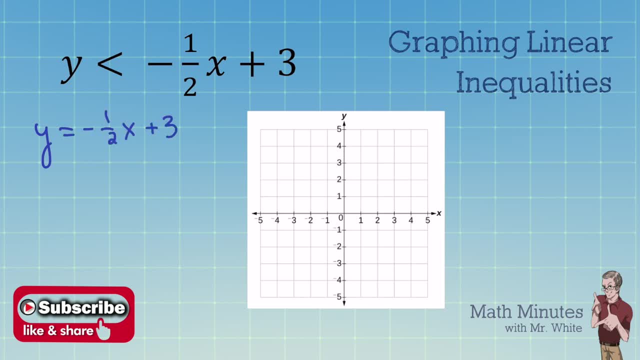 y equals negative 1, half x plus 3.. So we go up 3, put a dot From there, because the slope is negative 1. third, we're going to go down 1 to the right 2 and get our second dot. 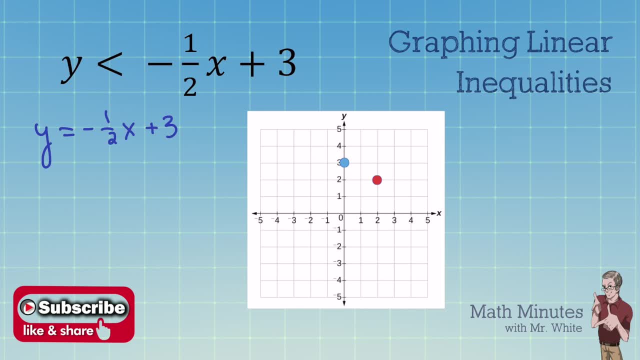 But this time, instead of drawing a solid line, we're going to draw a dotted line. It's a little bit like that open circle concept. when you were just working with you know, x is less than 3. You would have drawn an open circle. 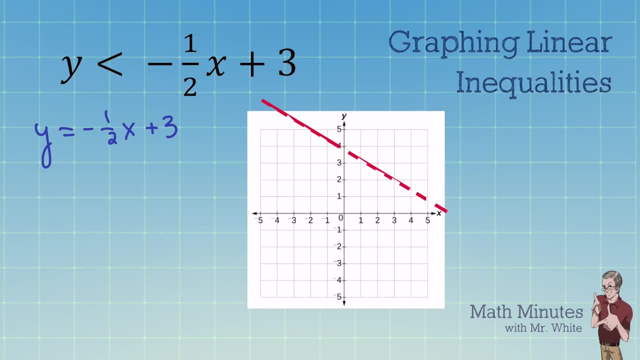 with an arrow to the left. This is going to be a dotted line to show that solutions are not on the line actually. Now, which way are we going to shade? This is y is less than So. my little trick says: whenever you have, y is less than the line. 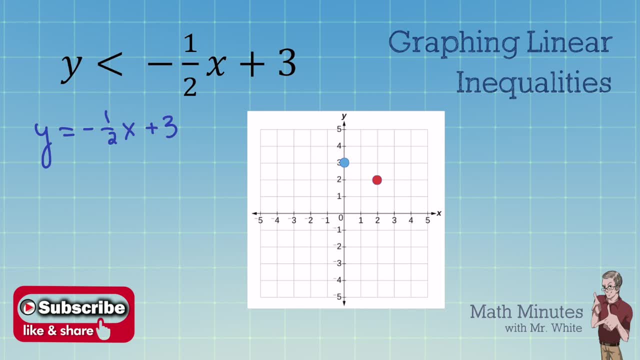 But this time, instead of drawing a solid line, we're going to draw a dotted line. It's a little bit like that open circle concept when you were just working with. x is less than 3.. You would have drawn an open circle with an arrow to the left. 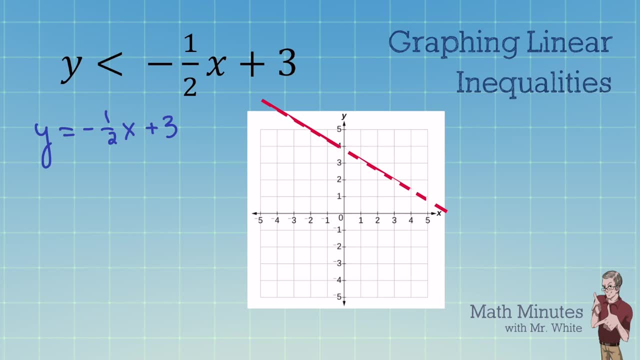 This is going to be a dotted line to show that solutions are not on the line actually. Now, which way are we going to shade? This is y is less than So. my little trick says: whenever you have, y is less than the line. 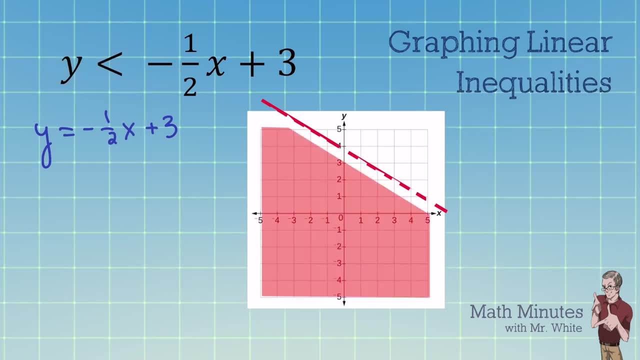 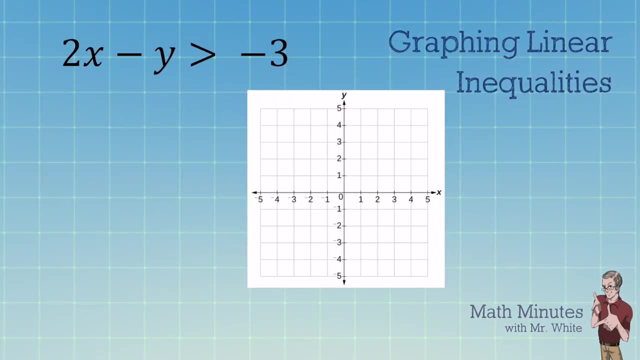 that means you go under the line, So you shade below the line. All right, one more example with another little twist. Whoa, look at this. This is set up differently, isn't it? This is not in. y equals mx plus b4.. 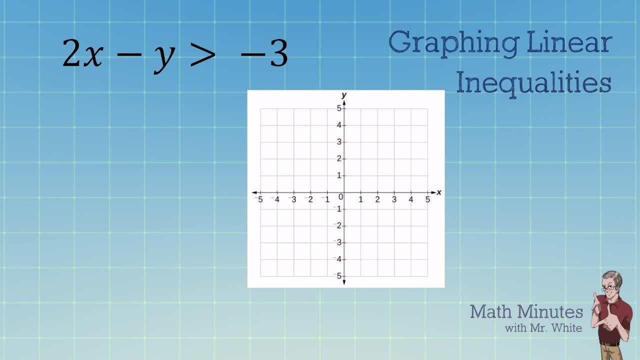 So I think that's the first thing I want to do- is I want to minus 2x on both sides. This is going to get me one step closer to being in. y equals mx plus b4. And then I got to get rid of that minus sign. 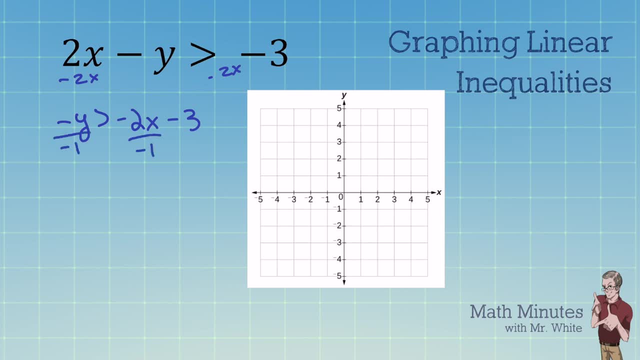 that's in the front. So I'm going to divide both sides by negative 1.. So everything gets divided by negative 1.. I now have y, I have 2x and I have plus 3.. Now be very careful. 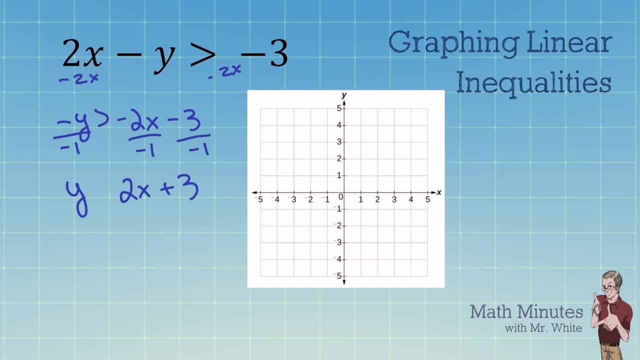 Do you remember this from algebra? Whenever you divide an inequality or multiply by a negative, you have to flip the inequality around. You have to flip that symbol around so it becomes y is less than the line. So let's graph the line. We go up 3, put a dot. 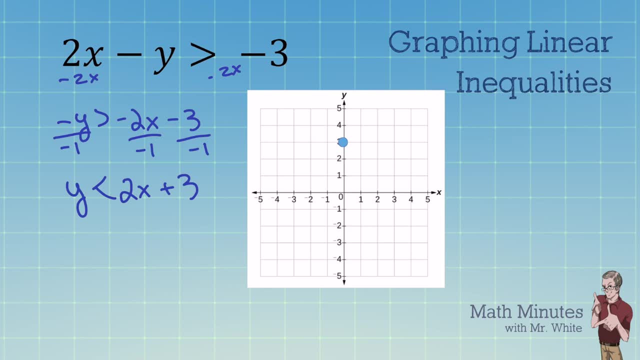 Then the slope is 2.. Now that's 2 over 1.. So we go up 2 over 1, get our second dot. But don't forget we're going to draw a dotted line because it does not have the equal part right. 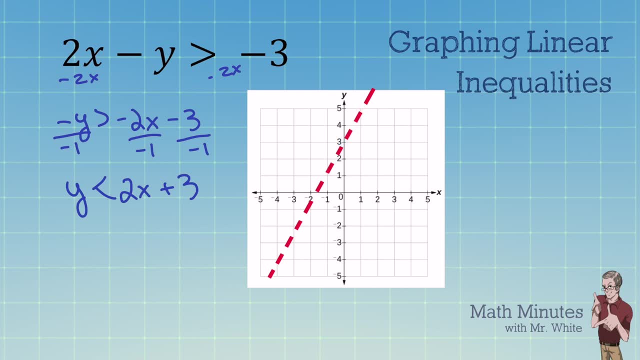 It's just: y is less than the line. Now we do have a less than symbol, so we graph under the line, We shade below the dotted line, and that would be our solution. region, Just to make sure you're clear on this. 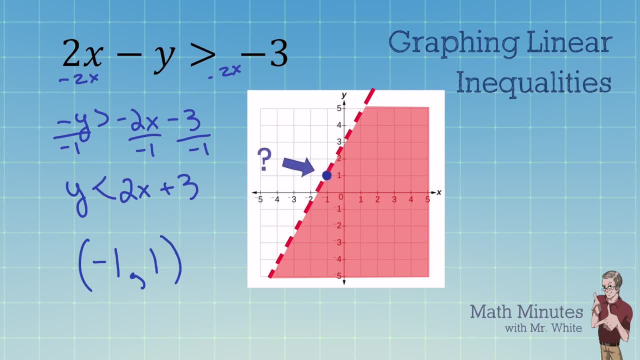 let me ask you a question: Would the point negative 1, 1,? would that be considered a solution to this inequality? Well, look at the graph. Look where it is. It's on the dotted line, which means: oh, it's so close. 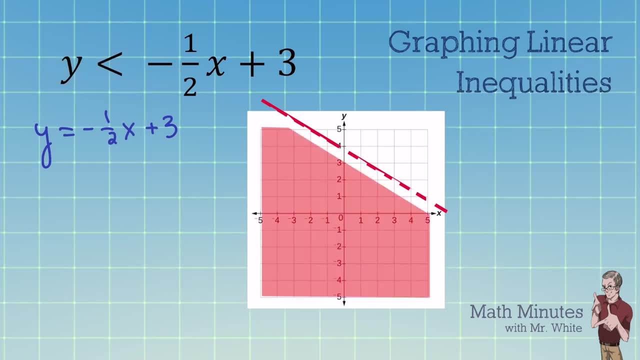 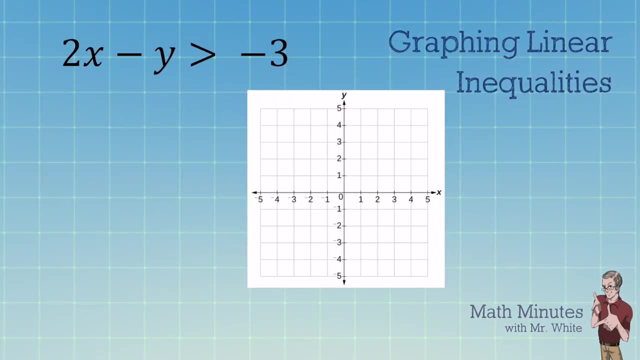 that means you go under the line, So you shade below the line. All right, one more example with another little twist. Whoa, look at this. This is set up differently, isn't it? This is not in. y equals mx plus b4.. 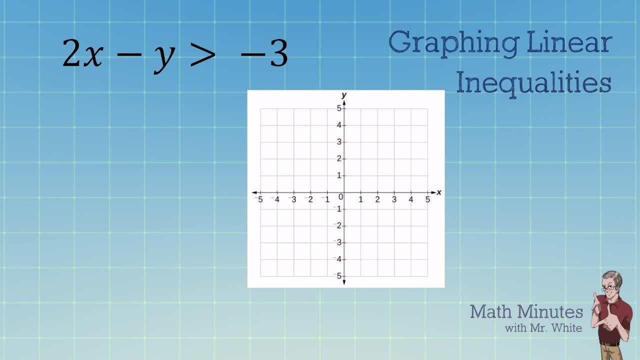 So I think that's the first thing I want to do- is I want to minus 2x on both sides. This is going to get me one step closer to being in. y equals mx plus b4. And then I got to get rid of that minus sign. 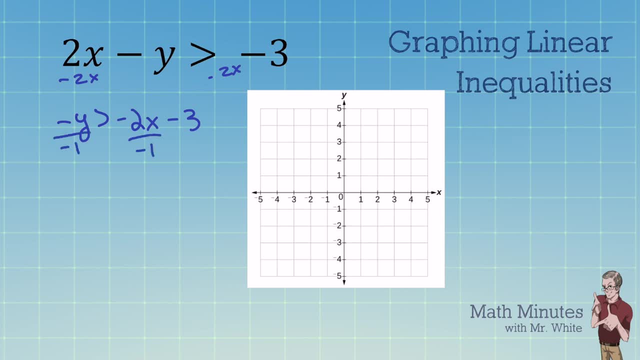 that's in the front. So I'm going to divide both sides by negative 1.. So everything gets divided by negative 1.. I now have y, I have 2x and I have plus 3.. Now be very careful. 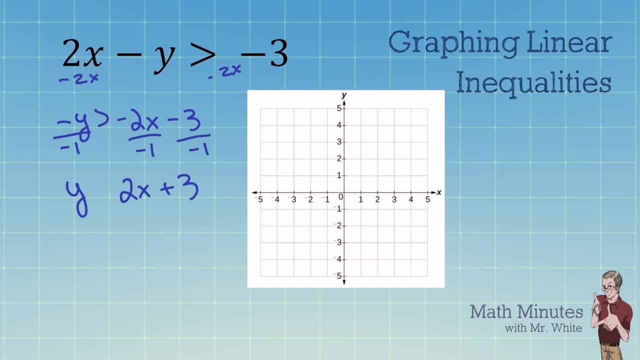 Do you remember this from algebra? Whenever you divide an inequality or multiply by a negative, you have to flip the inequality around. You have to flip that symbol around so it becomes y is less than the line. So let's graph the line. We go up 3, put a dot. 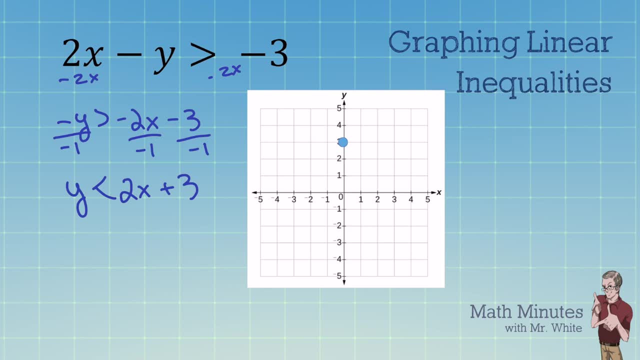 Then the slope is 2.. Now that's 2 over 1.. So we go up 2 over 1, get our second dot. But don't forget we're going to draw a dotted line because it does not have the equal part. 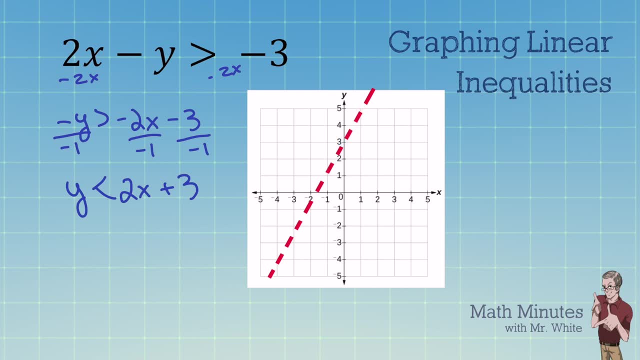 It's just: y is less than the line. Now we do have a less than symbol, so we graph under the line, We shade below the dotted line, and that would be our solution. region, Just to make sure you're clear on this. 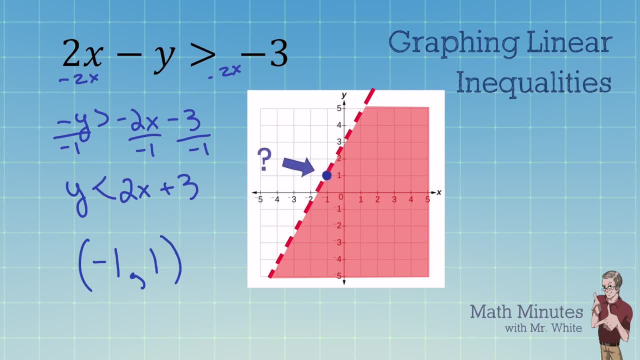 let me ask you a question: Would the point negative 1, 1,? would that be considered a solution to this inequality? Well, look at the graph. Look where it is. It's on the dotted line, which means: oh, it's so close. 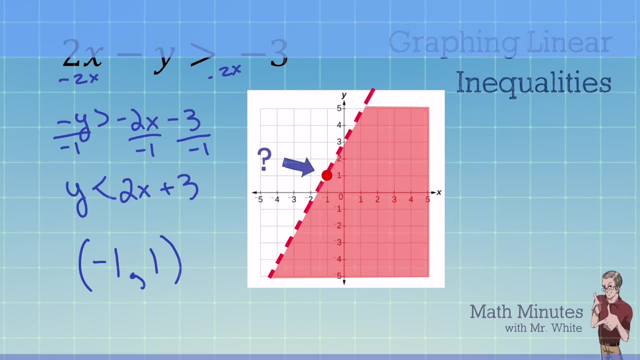 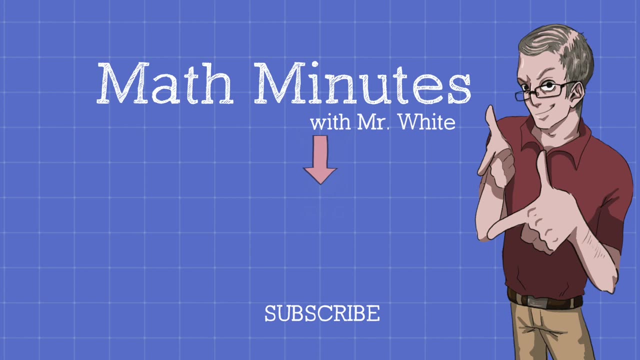 So it is not considered a solution here. Hey, if this helped you understand how to graph linear inequalities, leave your comments down below. Be sure to like the video and don't forget to subscribe to my channel. I really appreciate it. All right until next time.